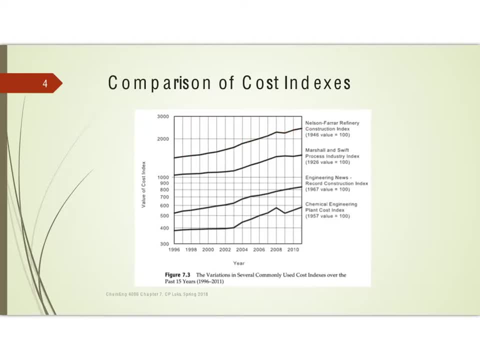 And the Nelson-Farrar Refinery Cost Index, And all of these have sort of the same general patterns, And so it doesn't make a lot of difference which one of these you use. You will get a similar trend, but the numbers will be different. 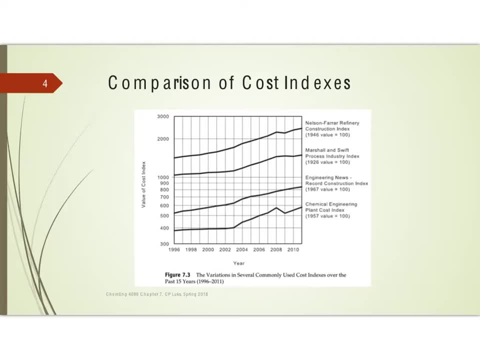 So you want to make sure you're always using the same index, No matter what you started with. stay with that one. Now, these were all started at different times, So Nelson-Farrar started at different times. Nelson-Farrar started in 1946.. 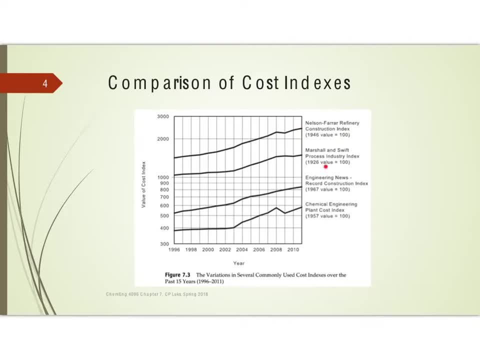 And that's when they set a value of 100.. Marshall-Swift started in 1926.. The CEPCI started in 1957 with a value of 100.. And you can see here in this picture that it's up over 500.. 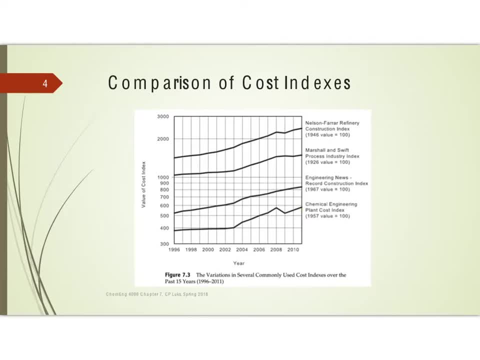 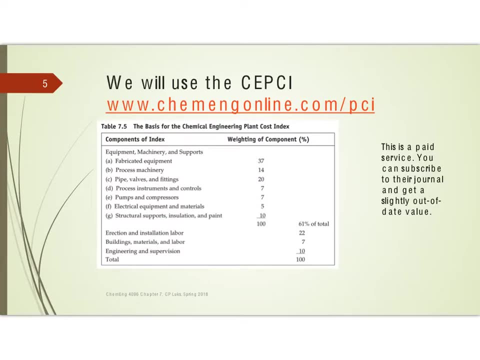 And in fact it's quite a bit over 500 today. Now for my course. we use the CEPCI. You can get this from Chemical Engineering Online, But unfortunately it's a paid service. But you can subscribe to the journal and get a slightly out of date value. 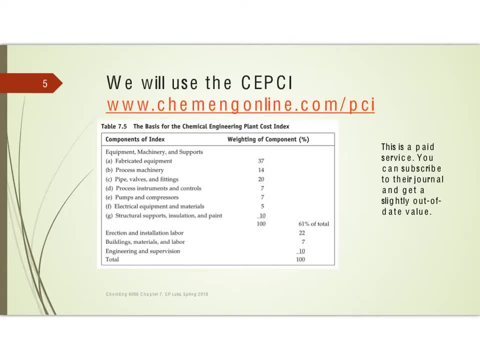 It's two months delayed And for the purposes of class that's more than adequate. But what the Chemical Engineering Online Magazine does is they look at these items here, So the equipment they're considering is the fabricated equipment. This would be things such as: 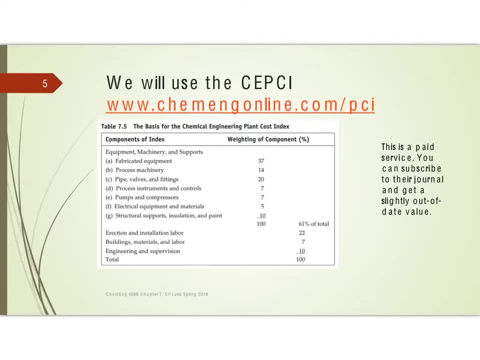 say, a distillation column, Something like that Process machinery. So maybe we're needing some filters or something. Pipes, valves and fittings, The instruments and control systems, Pumps and compressors, The electrical equipment and materials associated with that. 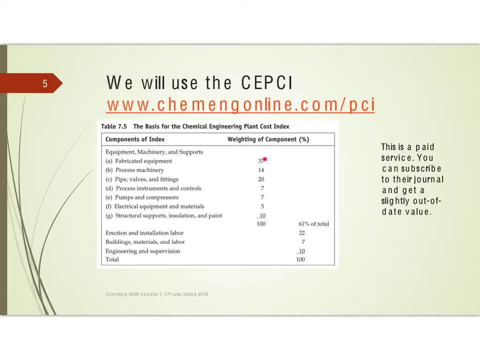 And then all of our structural supports And they're weighted relative to what is typical for building a standard plant. Then, in addition to the equipment, which is 61% of the total, they also look at installation costs, construction costs, labor. 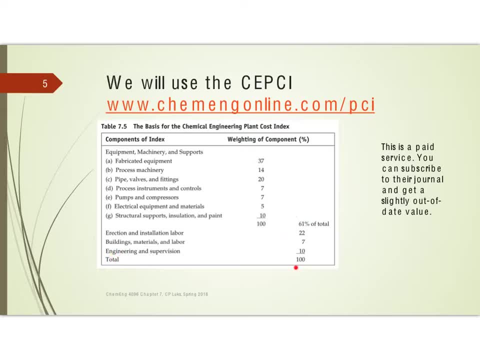 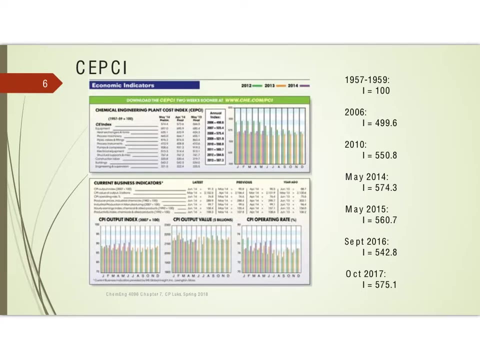 engineering and supervision costs, So that they come up with a total way of estimating this for the total amount you would have to pay to build a plant. This is an excerpt from the Chemical Engineering online magazine And it's always the last inside page of their magazine. 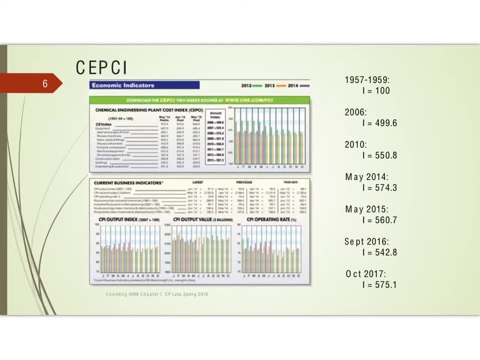 And they're going to show you various values. They're going to have recent values a year back. They're going to show you graphs over time And notice the years up here so that you can see that 2012 was really high and then it had come back down. 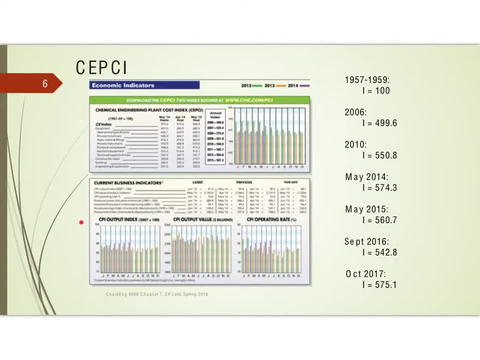 for instance, And then there's all sorts of other subsets that you might look at. down here We're going to use just the CE index, And you want to find the most recent, which you find it here Now. these are some values. 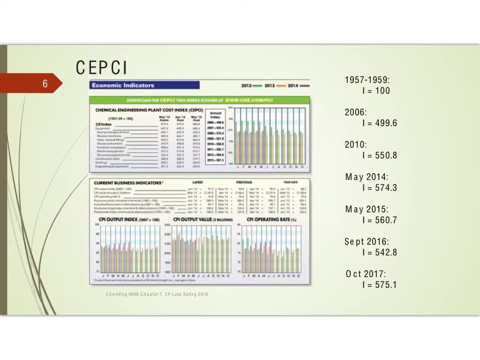 October 2017 was 575.1. The numbers change all the time, But you'll see that it's been a little bit stable over the past four years. It went down for a while and then it's coming back up. I always like to point out that. 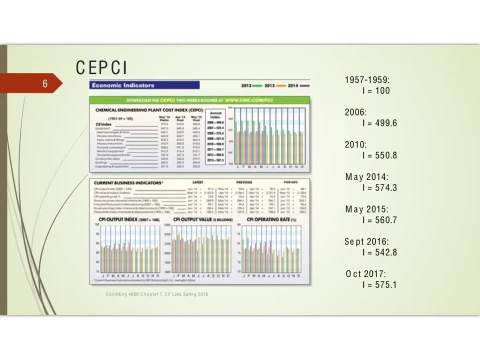 it's actually. really. this is a good predictor of what the economy is in our industry And sort of projects, a little bit about what your opportunities for finding a job will be. So it's a useful index to look at, not just for doing cost estimates. 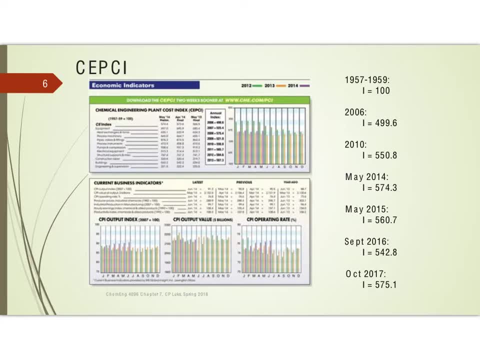 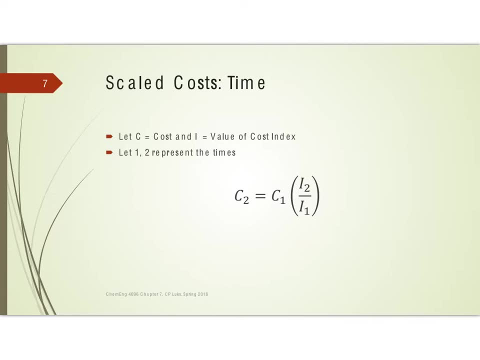 but also for predicting what the industry is doing in general. Now, the way of using these cost indices is actually very simple. It's simple ratios, No exponents, anything like that. So if you have a cost at time one, and you know the, 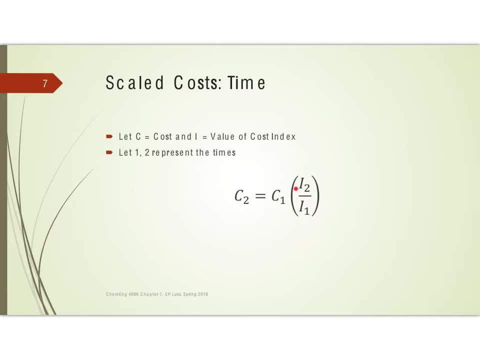 index at that time. you can look at the index for today and simply use ratios to come up with the cost for today. So let's look at an example. And so in 1993 a sedimentation tank cost $25,000 and we want to know what it would take. 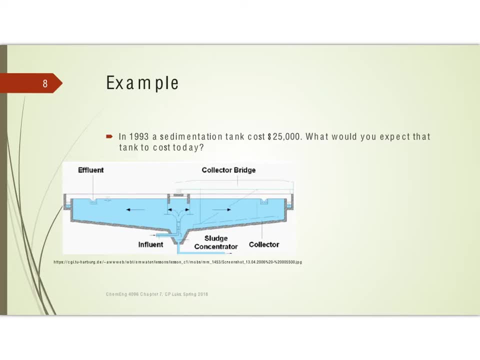 if we wanted to exactly replace that tank today. So there's not going to be any change in size. So the first thing we need to do is this is going to be cost at time one and I need to know the index at time one. So in 1993. 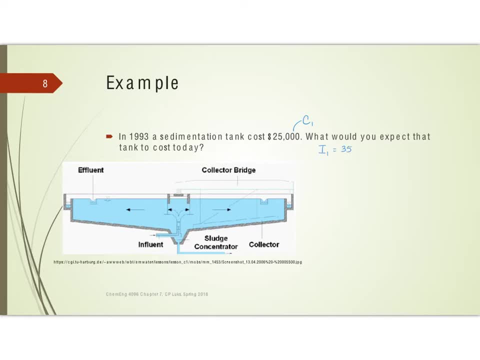 the index was $359.2, $359.2, $359.2 And if we use- and I'm going to just use 2016, just for simplicity- So So in 2016, So in 2016, the value of the CEPC was $541.7. 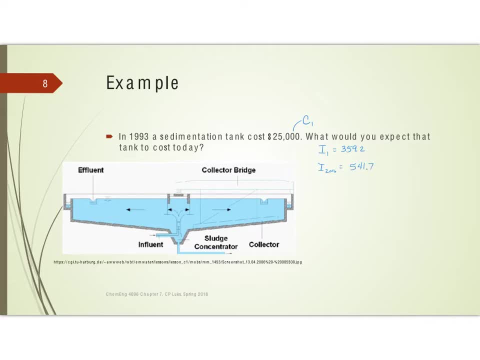 Now, actually, as I'm creating this video, it's actually quite a bit higher than that, but this is just to see how to work this, And so, therefore, all I'm going to do is to figure out what the cost is in 2016. I would take the 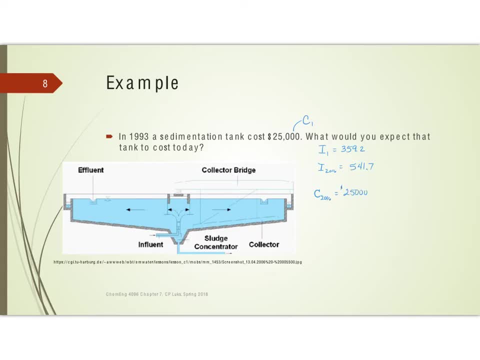 $25,000 and multiply by the new rate index over the old index, the old index, And if you multiply these out, what we're going to see is that we're going to again get some crazy number: 37701.83741648, 37701.83741648. 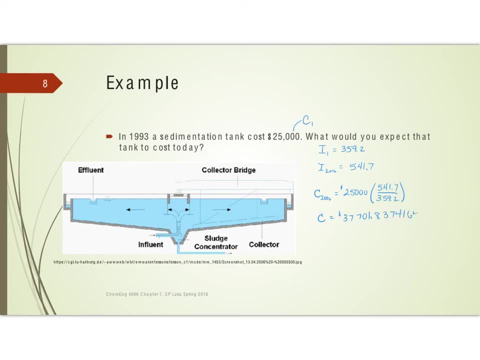 37701.83741648, 37701.83741648, 37701.83741648. This just keeps on giving, And so when we're doing this, because it's a cost estimate again, my rule of thumb is: I on preliminary numbers before I get to the. 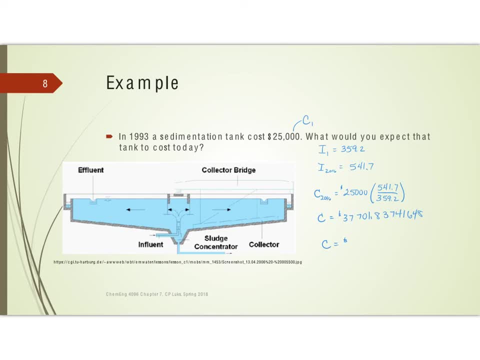 final project total. I'm going to always keep one extra digit, and so $37,700 is a good estimate for the sedimentation tank today. So in our next lesson, what we're going to do is we're going to look at a project where I have data. 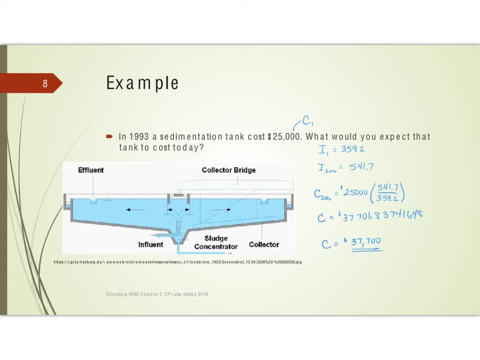 but the size and the time have both changed. Thank you very much for your time.